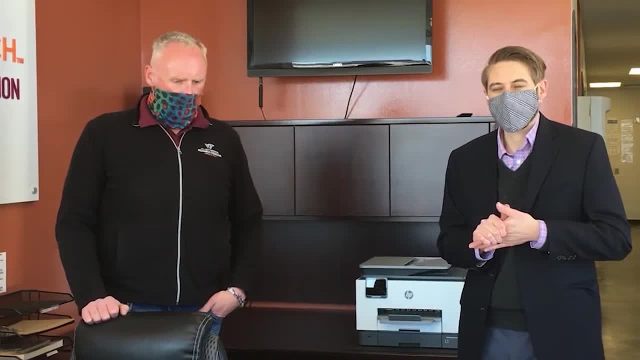 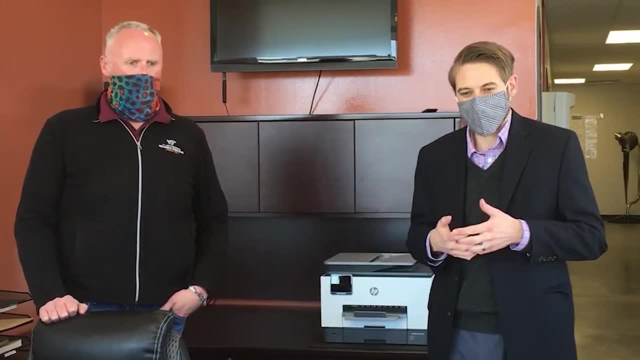 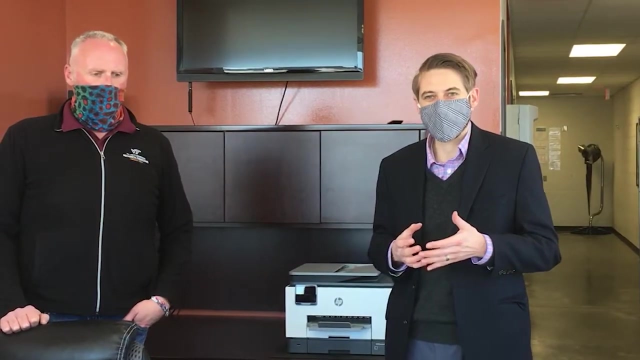 was a renewed push at Virginia Tech for propulsion related research and part of that push was because of some industry commitments. so I wanted to just mention we have a couple of industry focused partnerships. one of them is with Pratt and Whitney. we have a Center of Excellence at Virginia Tech and then the 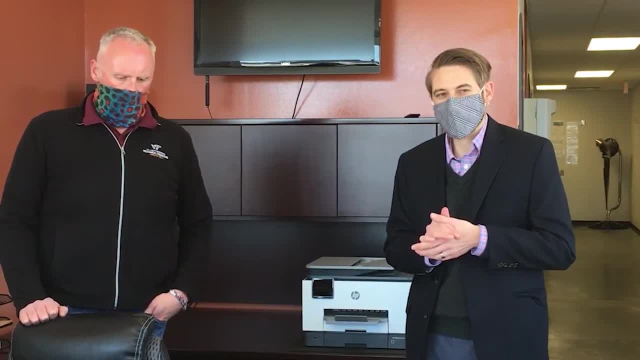 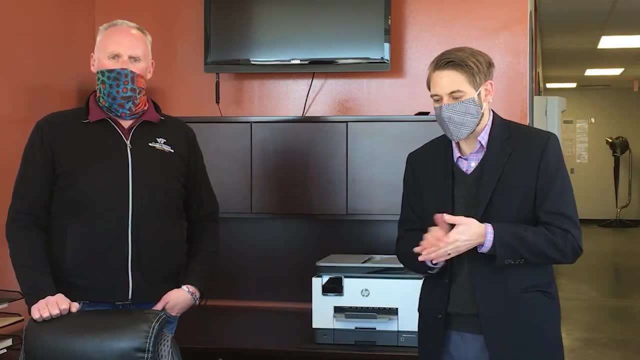 other thing that was happening- it was really important about that time I was mentioning- was a relationship with Rolls-Royce, and so, if you don't know, Rolls-Royce makes aircraft engines and marine engines and things like that, but really their aircraft engines division that had approached Virginia Tech and 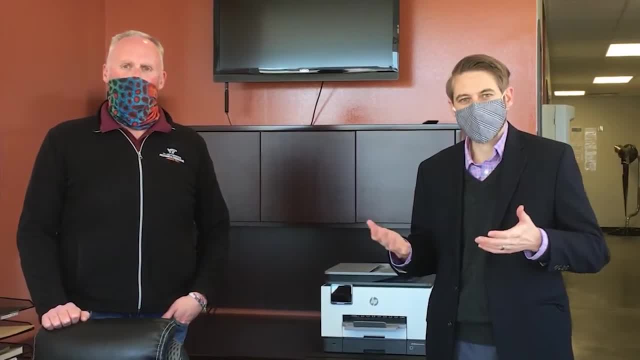 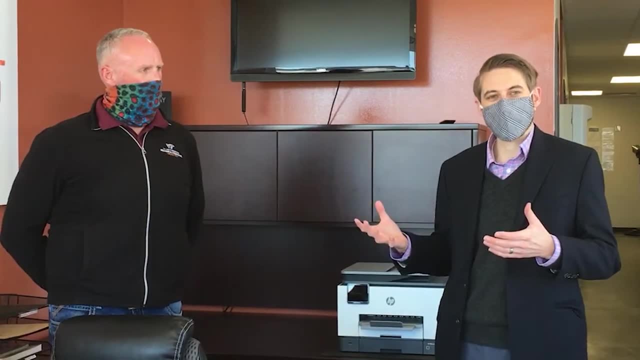 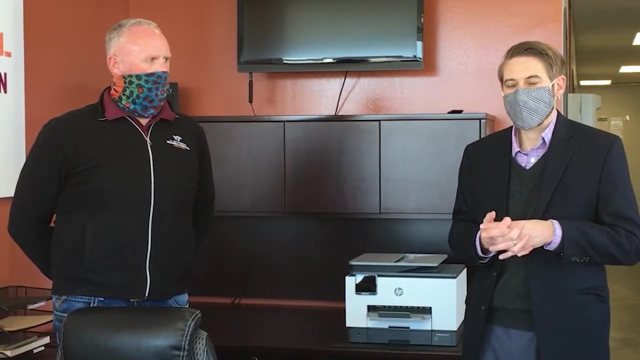 there was a lot of momentum with getting work going here, and so about that time that we began working with Rolls-Royce, there was also this, this opportunity through the College of Engineering to build this laboratory, and I think, one of the things to point out, as Eric mentioned a minute. 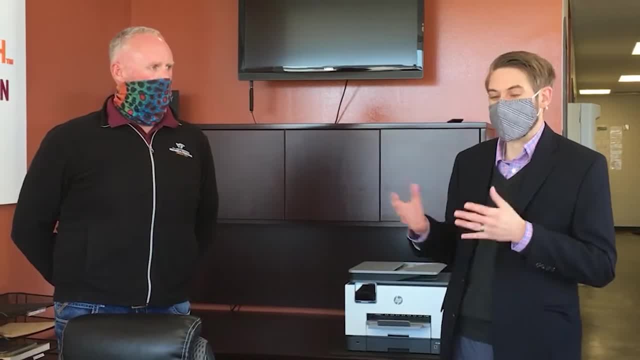 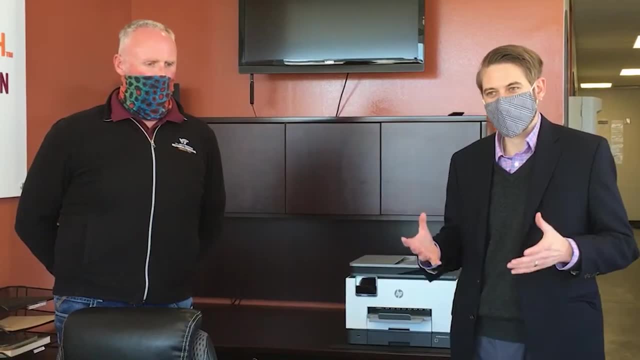 ago is that there's seven faculty members. these are not just faculty in aerospace and motion engineering, they're also mechanical engineering and really this laboratory represents a college level asset. so it's a really big deal in the college and it's giving us a lot of capability. 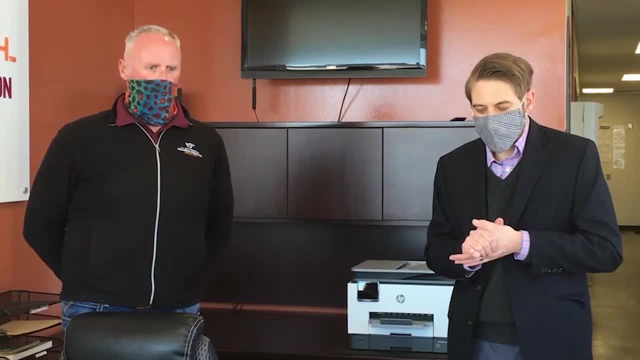 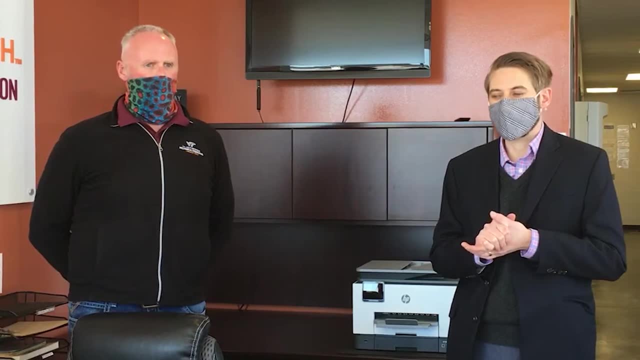 to do propulsion focused research, so to speak. to that then I've already mentioned two of their very important industry partners. there's several others that I've not mentioned. we also do lots of research for the government, so office of naval research is a really big sponsor office, Air Force, Office of 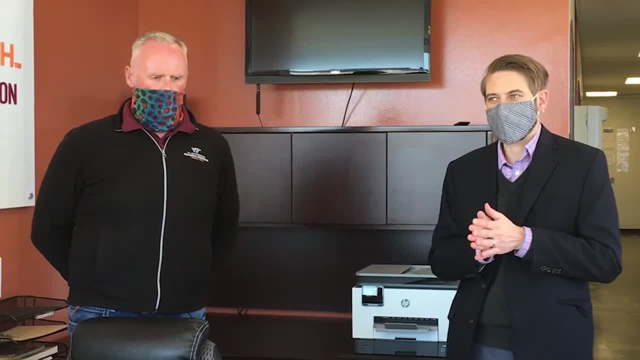 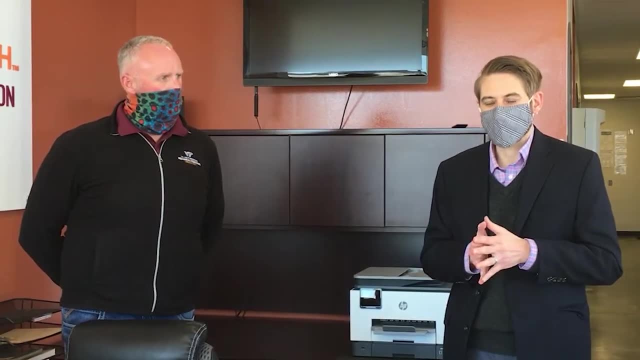 Scientific Research. there's also a little bit of work for the Army, some work for the Department of Energy, and I'm sure I'm missing some others as well. so pretty diverse portfolio of things that are going on in the industry, and I'm sure I'm missing some others as well. so pretty diverse portfolio of things. the 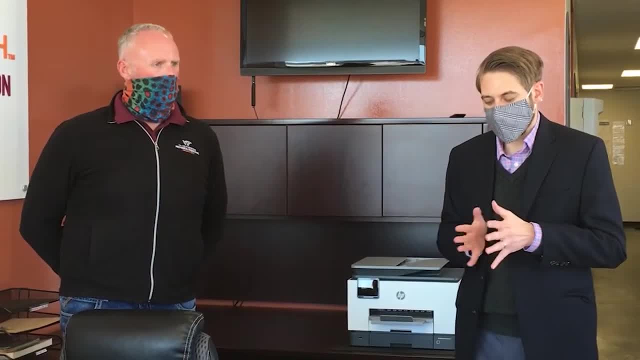 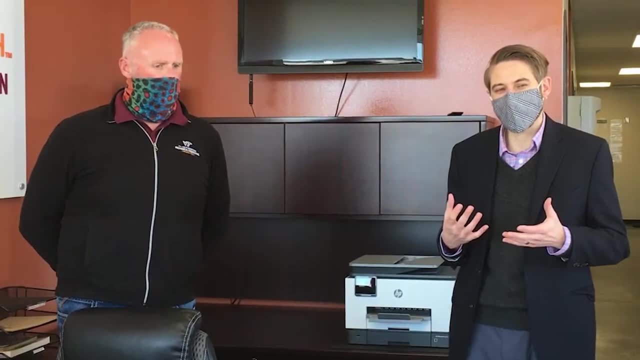 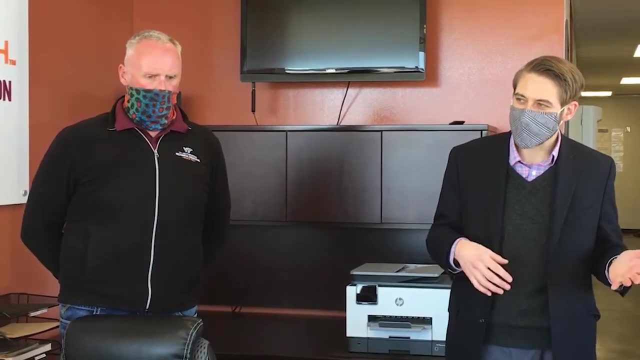 go on here. when this lab was originally built, it also looked at some of the synergies and advantages that we had at Virginia Tech. so one of them is that we operate full-scale, full-size gas turbine engines, not for test or not for certification, but for research. so one of the really cool, I think, things that we 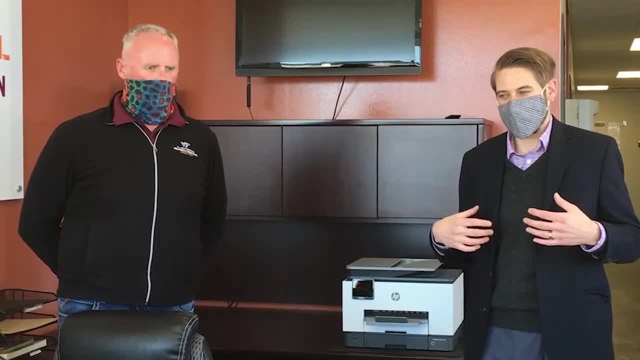 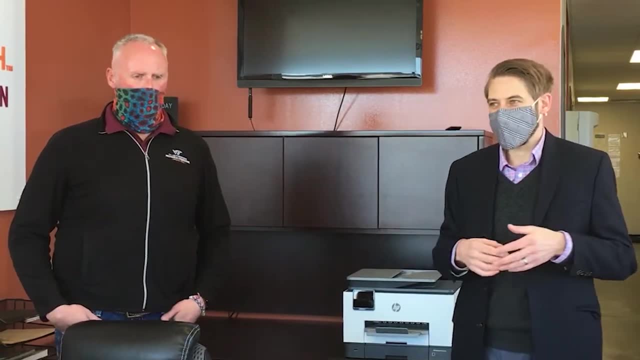 do is that I can be in my office on campus, think of a crazy idea, of a new way to measure or something let's say, and then I can do that. so that's great, Thank you very much. can propose that to someone in the government. We'll come over here and use. 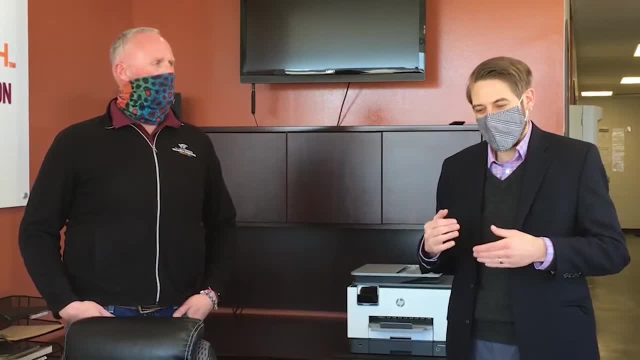 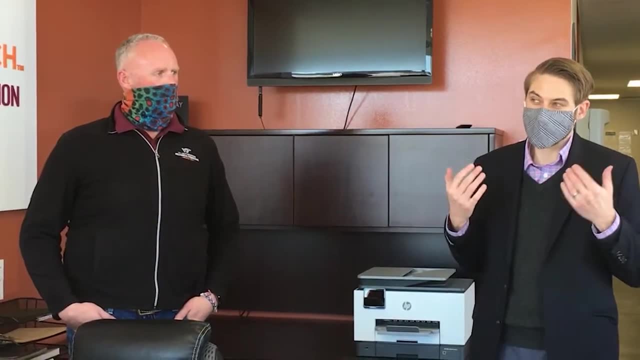 some of the small laboratories to prove out the basic idea, and then we can take that idea and we can apply it on one of the rigs I'll show you in just a minute. After that it gets exciting enough that we say, hey, let's try it on the engine. 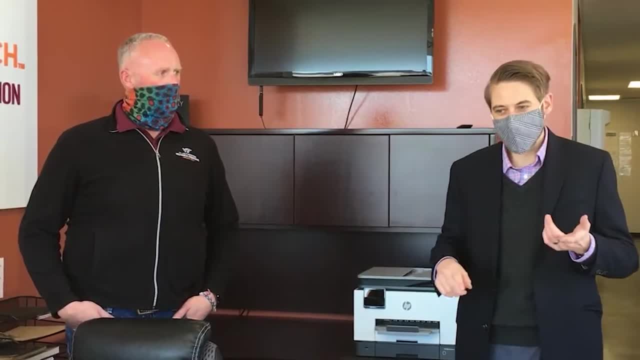 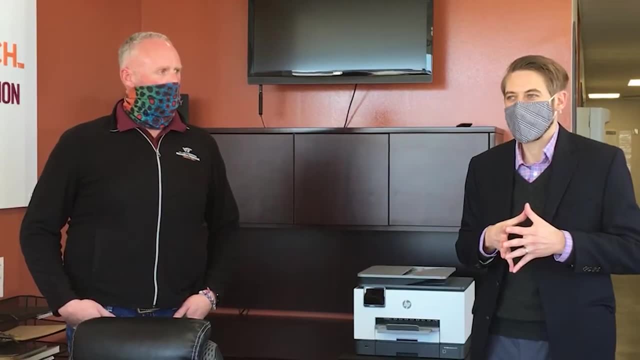 and at that point we're already working with, let's say, the Navy and also maybe Rolls-Royce or Pratt & Whitney, in order to see a pathway to actually use that on a real system. So the thing that excites me about APPL is that we really go from 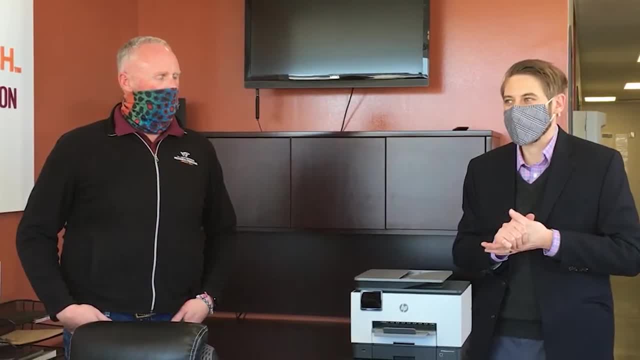 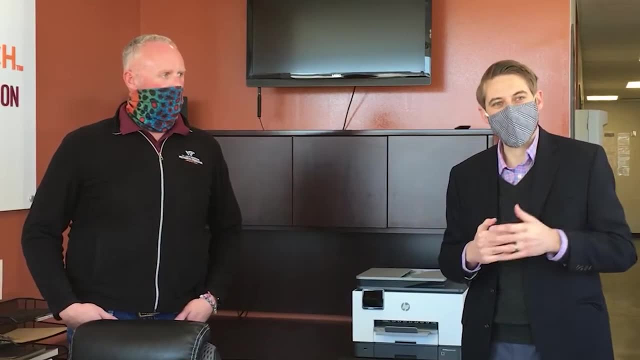 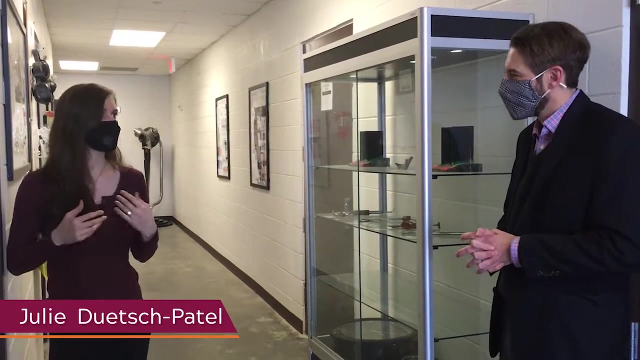 the very basic idea all the way to impacting the products that are out in the field, And so I think what you'll see in this tour are some of the capabilities that help us to scale that and to reach those different levels. What kind of things can you get made in the machine shop versus what would you need to outsource for a project? 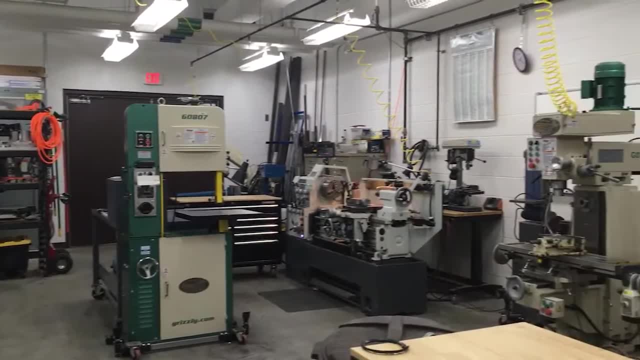 There's a pretty large array of different jobs that we can actually take care of. There's a pretty large array of different jobs that we can actually take care of. There's a pretty large array of different jobs that we can actually take care of. 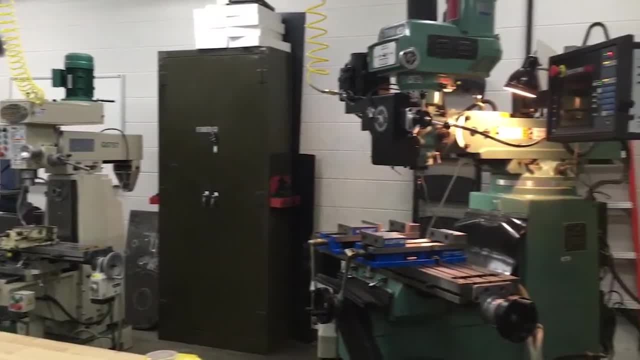 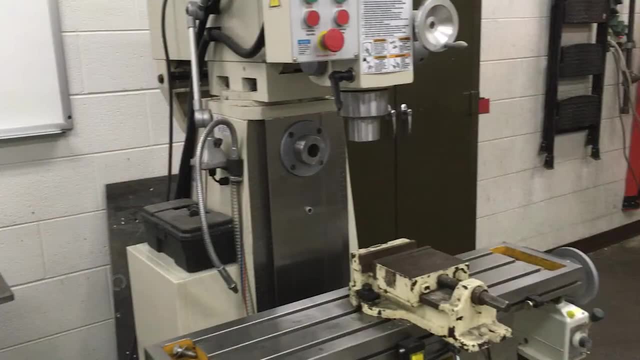 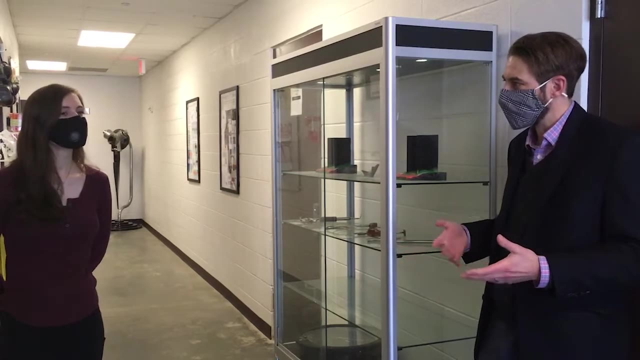 here at the machine shop. So the limitations really come down to. if you need to do very large pieces, all right, so that would be something that we just don't have the fixturing maybe to hold, or there's certain types of exotic metals that are really tough to hit the machine. Having said that, the 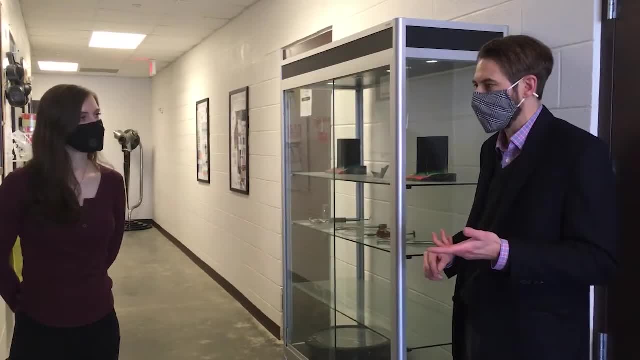 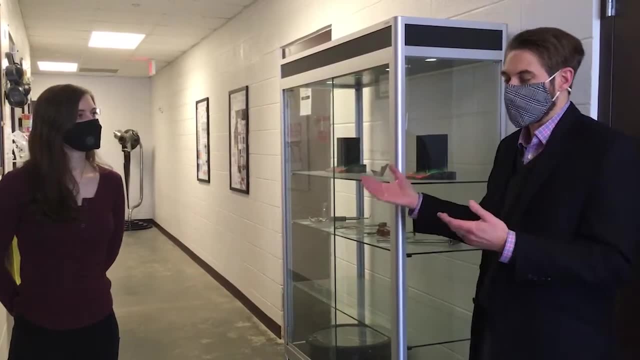 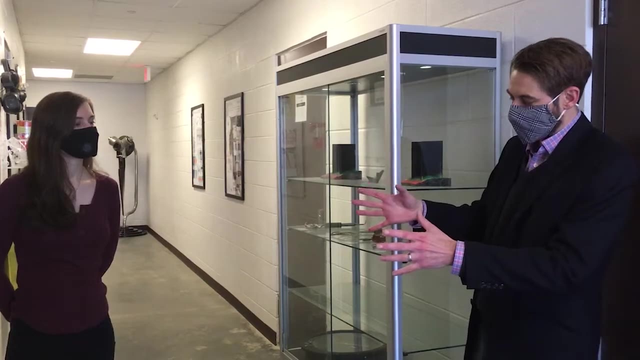 capabilities are quite broad. There's welding capability here, machining, milling, lathing. So one of the great things for the students is you're running the experiment here. you really need to get your results. something breaks all of a sudden Or you realize that when fixturing this, you 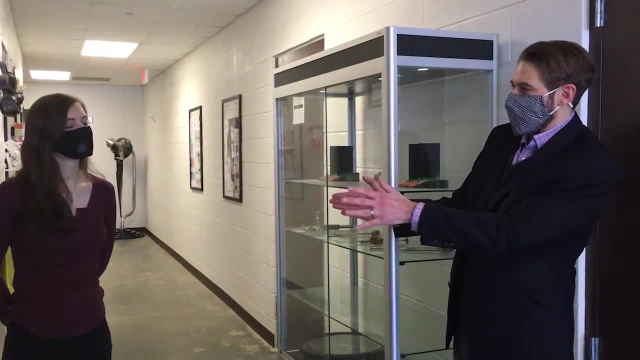 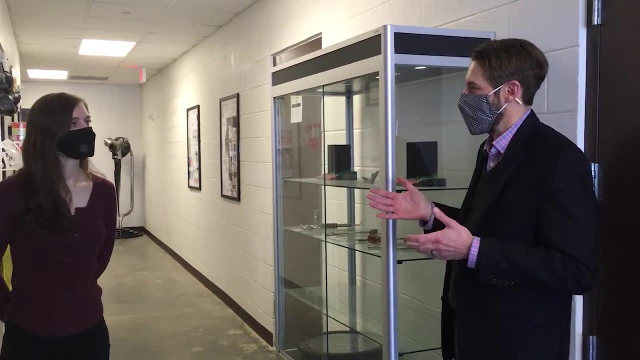 would love to be in the wind tunnel an extra half-inch downstream. So how do you do that? You need a little slot, let's say So. you come to Randall and he is really an agile professional that can come in, alter your hardware, have you up? 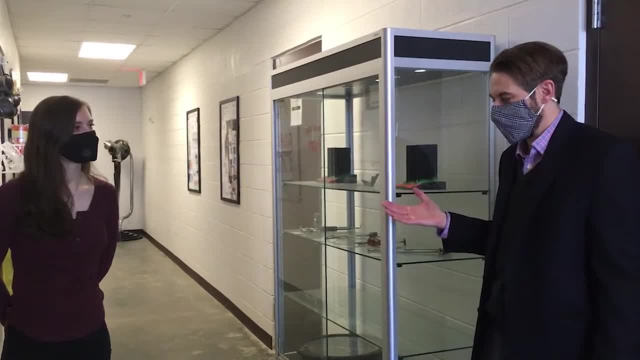 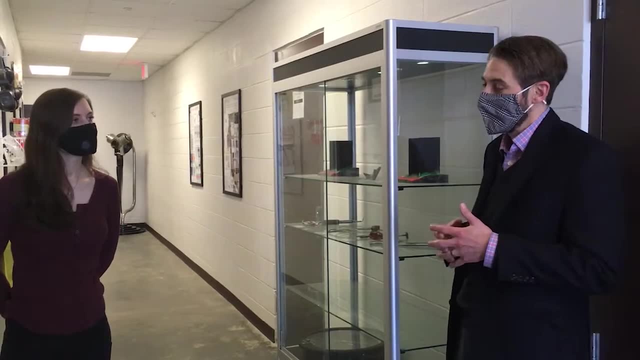 and going quite quickly, And that really covers everything from really simple apparatus all the way up to things that we do in the hypersonic wind tunnel. It could be highly, highly precision. So I think the answer to your question is: there's a wide array of things that we 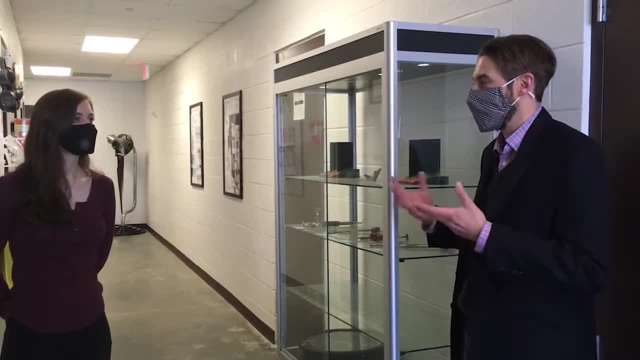 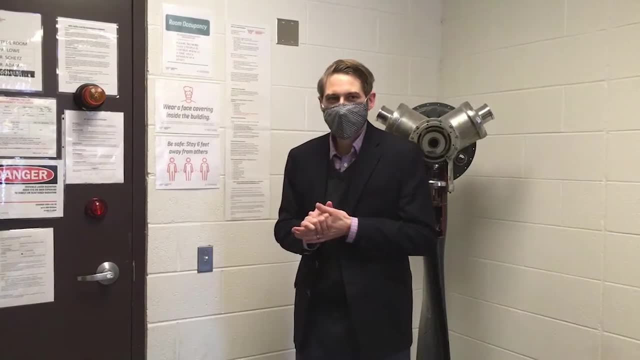 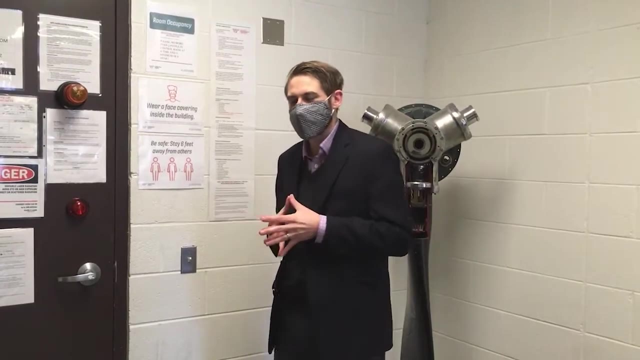 do, and just if it gets a little too large, then in that case the beauty is we do have a lot of really great local machine shop. We're standing outside right now of one of our most active laboratories. There are two very active rigs. There's one is a preheated supersonic jet. We use that for all for. lots and lots of types of research. It was originally built to study supersonic jet noise and find ways to reduce that. There's another rig that's getting lots of use now. that's a hypersonic wind tunnel. The hypersonic wind tunnel will go up to Mach 7, and so it can do that. 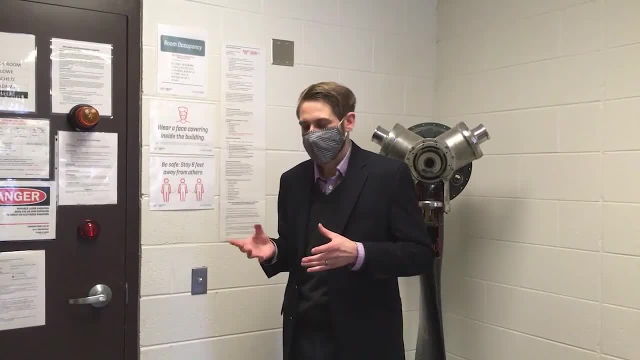 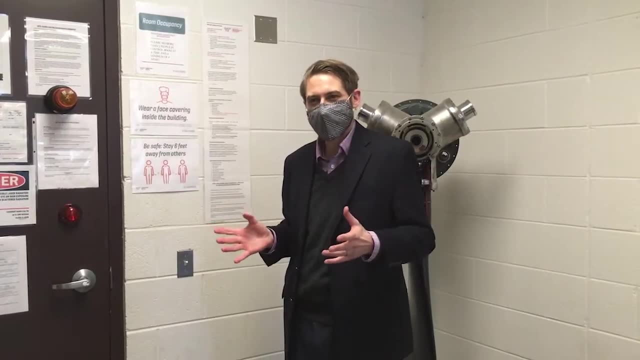 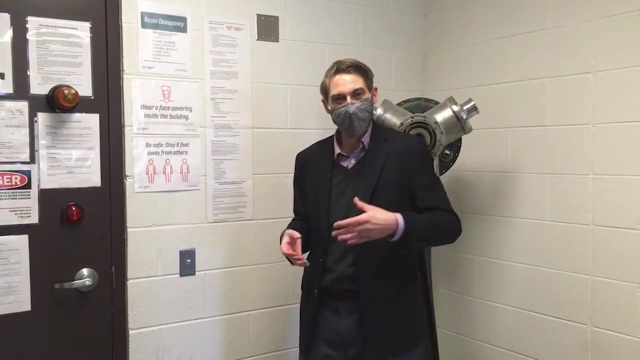 anywhere from Mach 2 up to 7, depending on which nozzle is swapped in, And so anytime you visit Advanced Propulsion and Power Lab, you might see a different set of rigs that are set up and ready to go to conduct research. This is very important for us to be agile in order to meet the needs of our 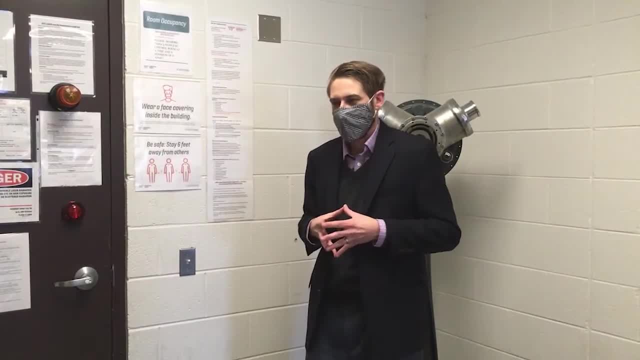 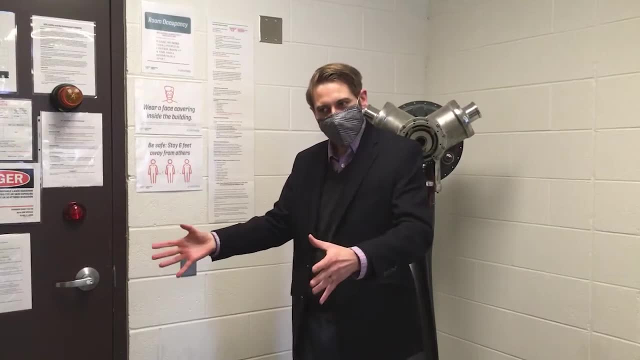 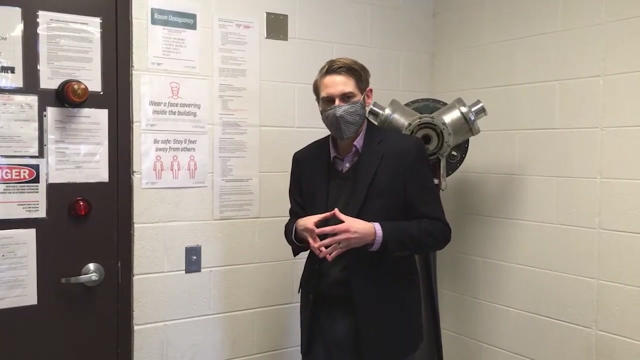 industry customers, also our government sponsors, And so the rigs that you'll see in the lab in just a moment, there are actually wheels on. the supersonic free jet rig allows us to move it in and out. that can make space for for other experiments, and this is copied throughout our entire laboratory. So it's 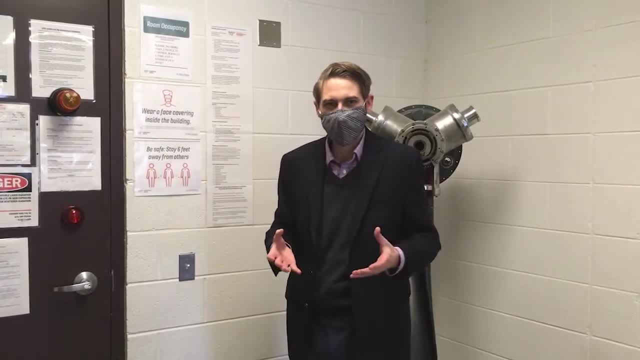 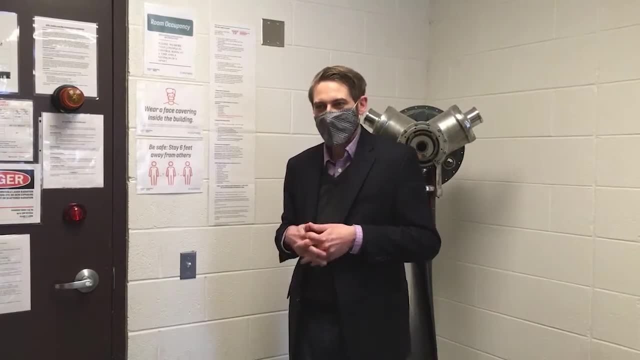 really about doing research agilely and if you were to come here and do research here, it gives you a lot of information. It gives you a chance to build your own rig and build in a modular manner that you can get really amazing data and use some of the resources that we have here in the 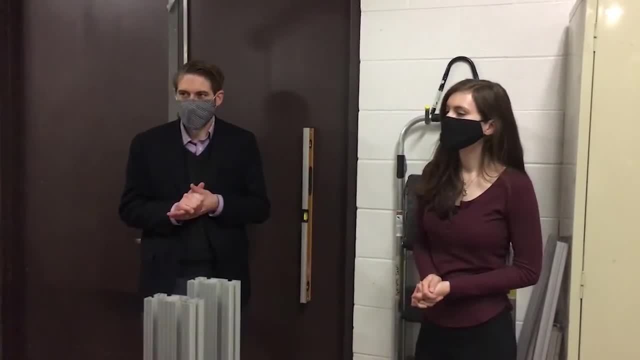 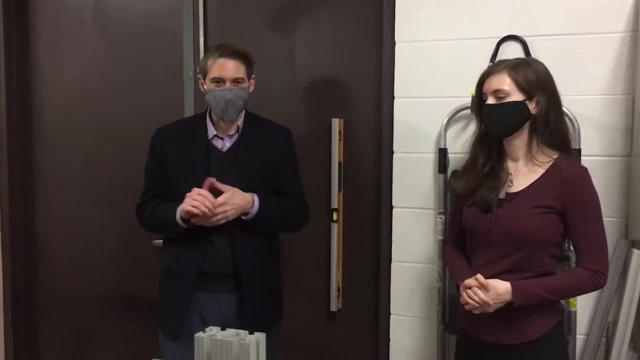 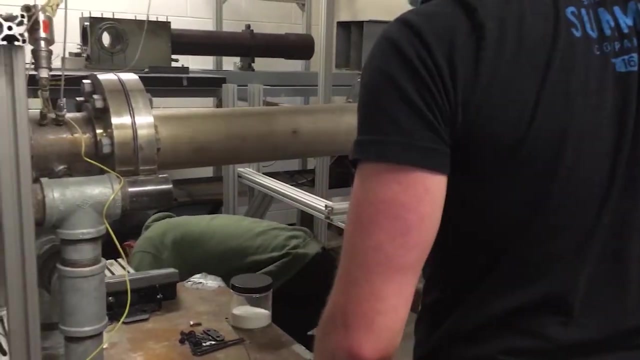 facility, Great. So we're now standing in this very active test cell I was talking about. In fact, it's so active that we have folks who are working right by me here on the supersonic free jet that I was just mentioning, And there's also the hypersonic tunnel further over to my right. 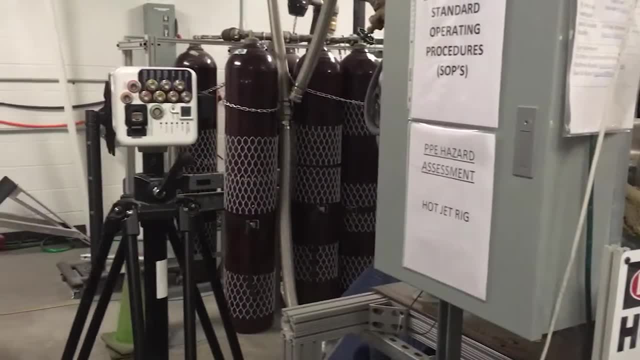 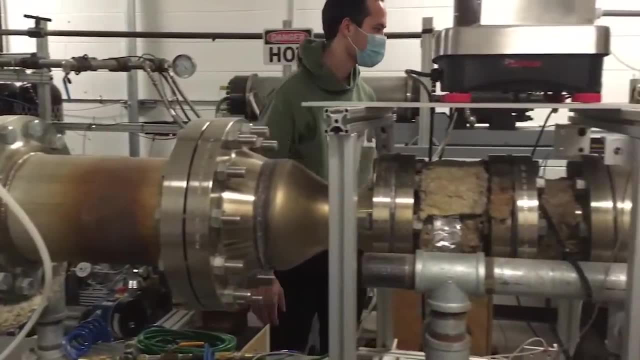 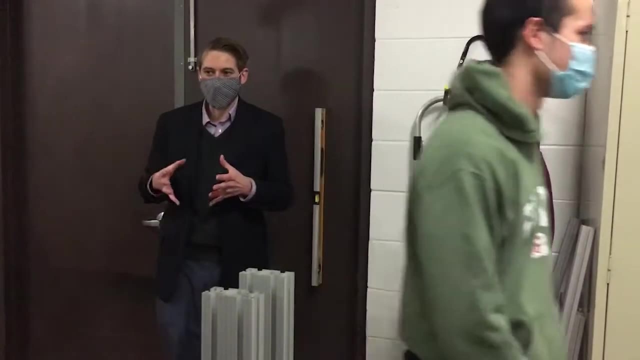 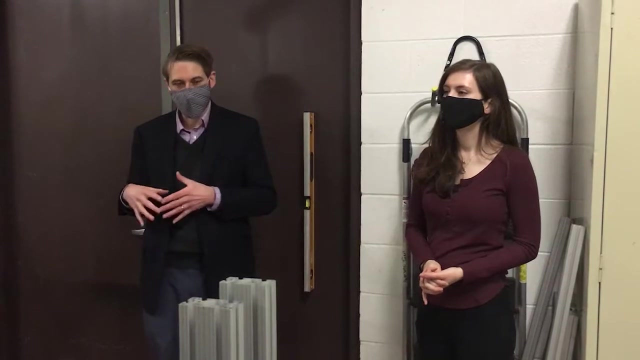 And so these rigs I was always mentioning are extremely modular and any time there is going to be some other experiment, that's set up, And this is all by design. It's really what we hope to have happen. There's activity in this room virtually all year long. This can happen anywhere from very short entries where people may come for a week. 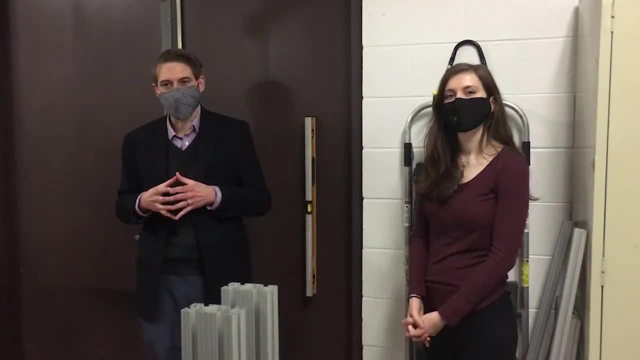 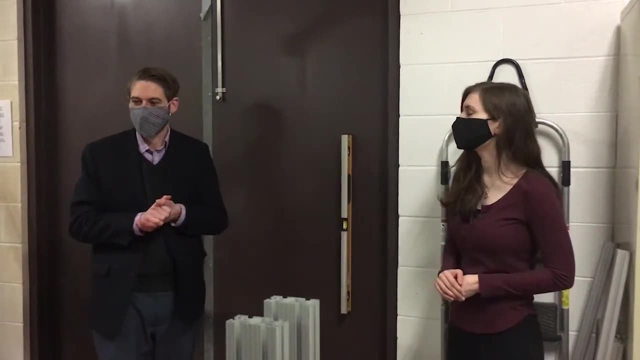 Up to folks who set up for, for instance, there were projects that will come, questions that were put in for jobs project lasted all summer but people were using the hypersonic wind tunnel. Well, you mentioned that this rig is modular. What kind of configurations have you run it? 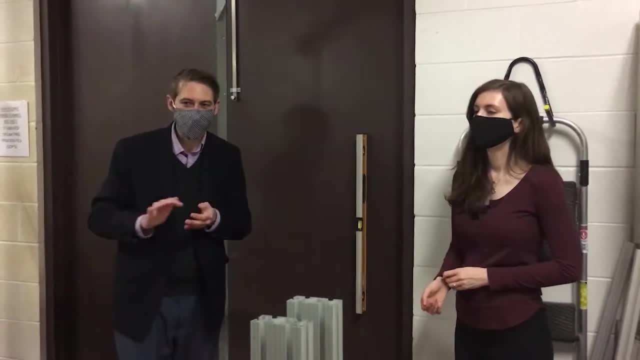 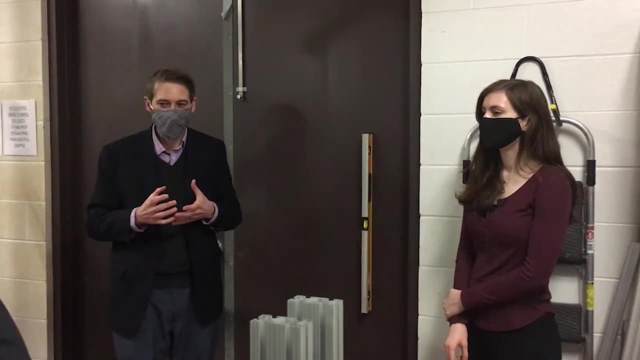 in for Absolutely So. the supersonic free jet I mentioned was built to study supersonic jet noise. It turned out to have a lot of other uses, And one really interesting that I'll bring up was that the Navy was having some trouble with. 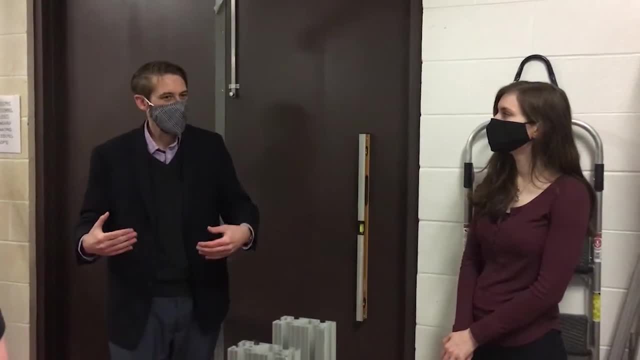 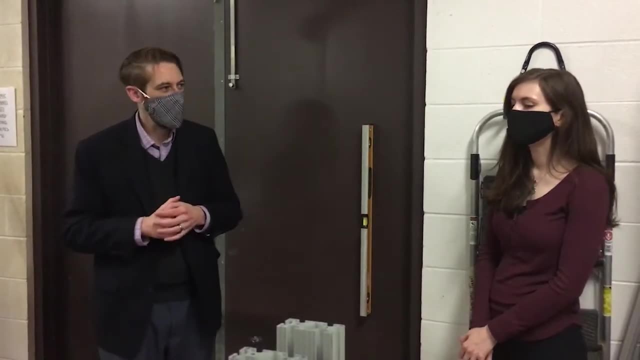 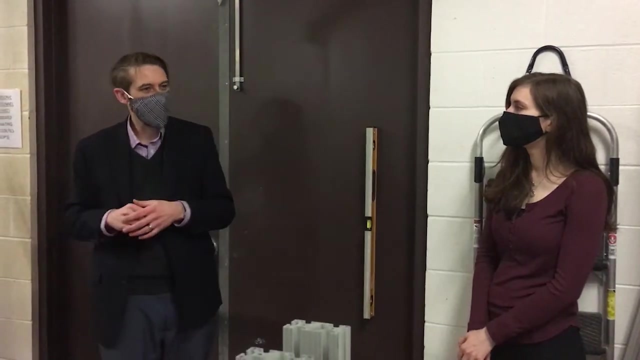 the deck of aircraft carriers, not understanding the heat transfer coming from the V-22 Osprey to the Navy slashing rings, And so I actually worked with a smart scholar who was here at Virginia Tech who used a corrugated deck panel from the Navy that then they placed that. 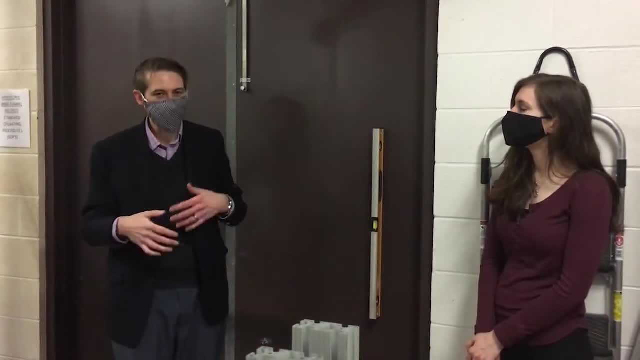 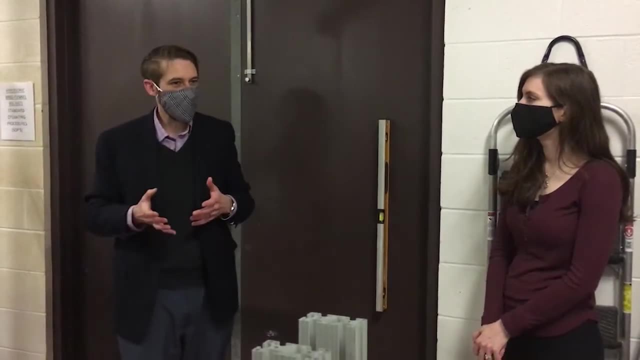 by this jet, which provided convective heat loads that we showed with the same heat loads that the V-22 Osprey provides, And then we made all the temperature measurements, etc. using basically some of the same sort of hardware. Another good example is actually: 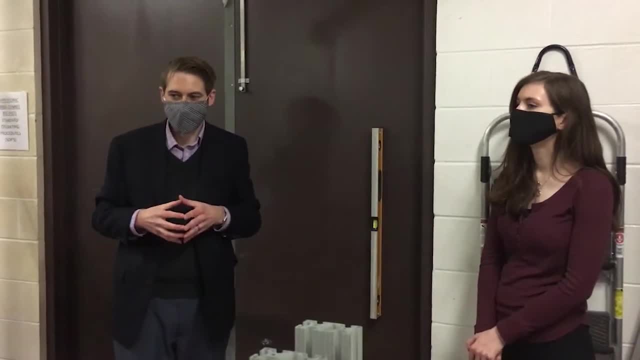 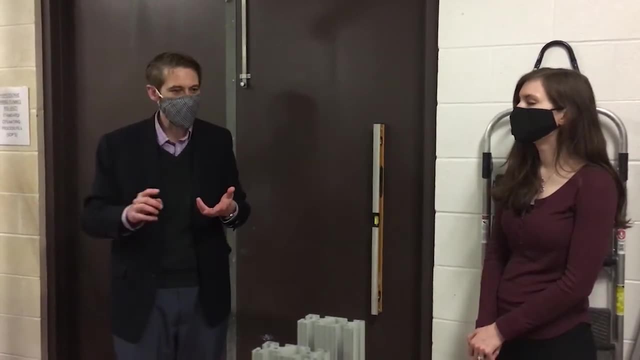 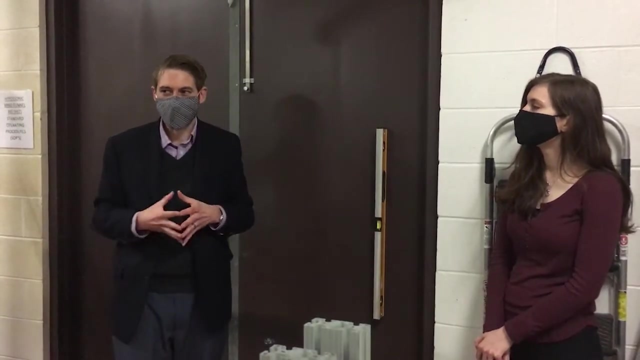 an approach set up here right now is that we use this same jet to look at the performance of sensors: temperature sensors, The current one is a particle concentration sensor, velocity sensors, pressure sensors, So there's tons of different uses of this. We really think of this rig as being a hot. 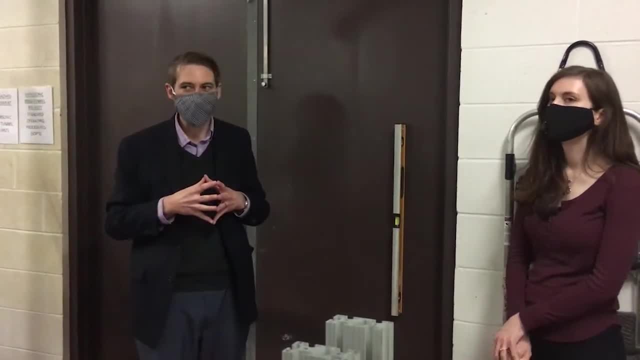 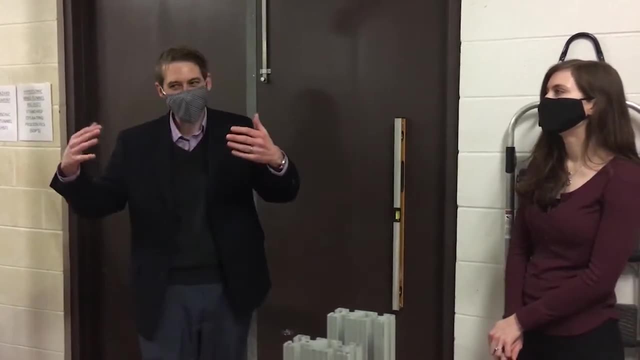 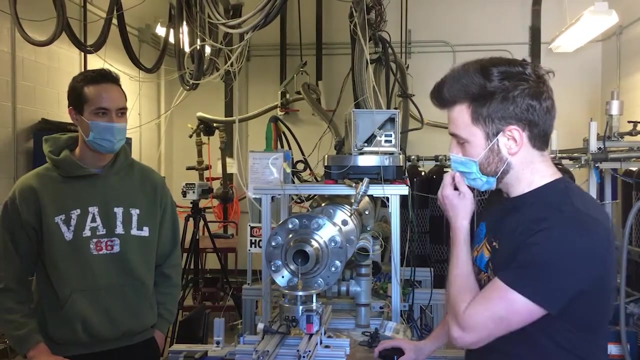 gas generator. There's an electric heater that's connected to it that anyone can use as a user of this facility. It provides 192 kilowatts of heat, and then we can use that high pressure hot air in our engine room. Hi Well, we're modifying this rig so that we can. 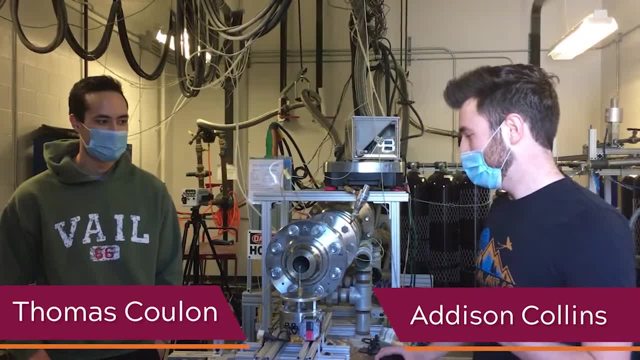 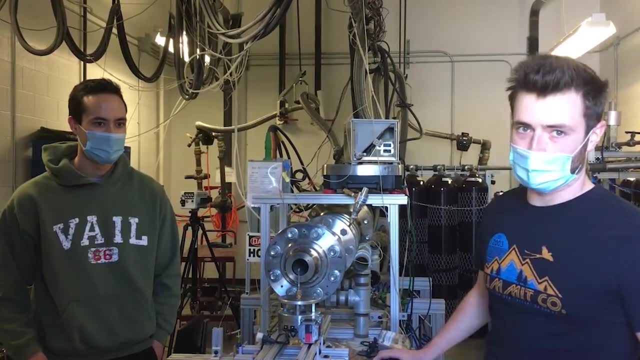 accelerate particles up to about 0.75.. And we're going to be using glass beads and they're going to enter a probe and we're trying to characterize this probe such that when we stick it in an engine later, we'll understand the values. 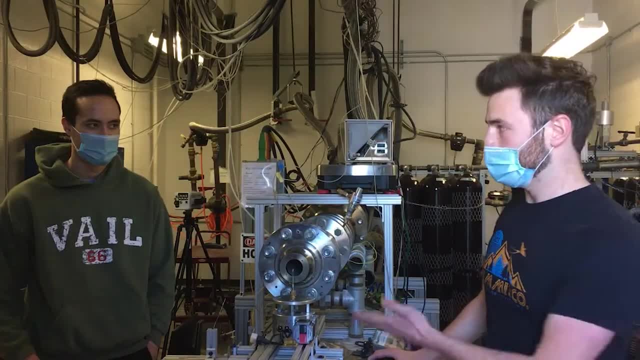 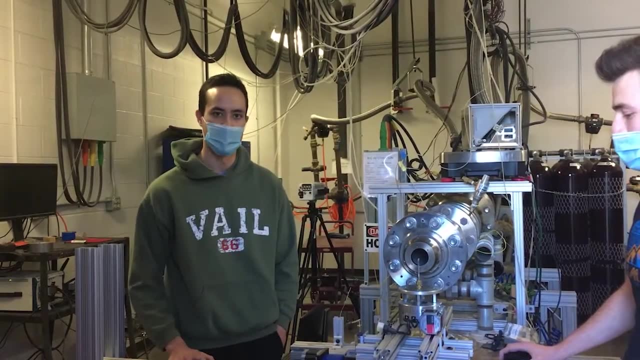 of the measurements we're getting And we'll be using SAM for that in the future, And Thomas will talk more about our blowdown or our shakedown program. Yeah, so right now we're basically preparing a new what we call blowdown for this coming Friday. 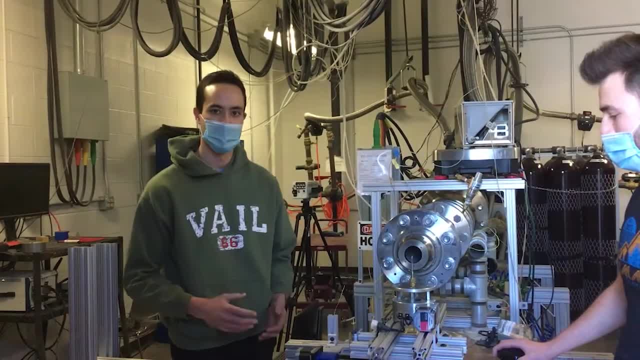 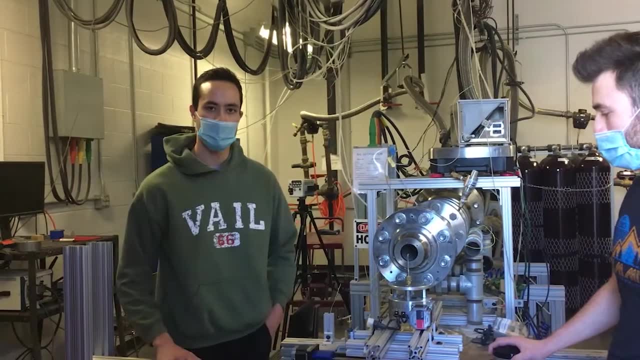 Basically, what it's going to be is: we're not actually doing our experiment, but we just want to make sure that everything works properly, that we know how to run the jet, that our probe can sample particles properly, And so that's what we're preparing for right now. 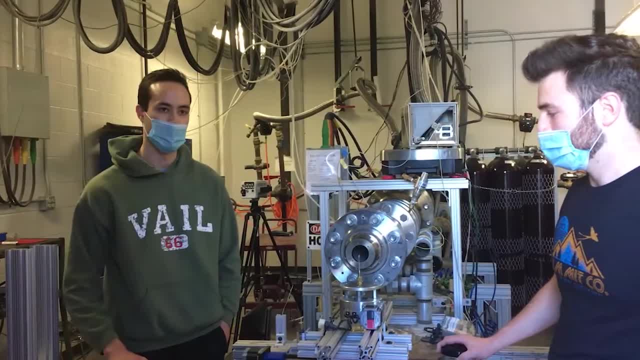 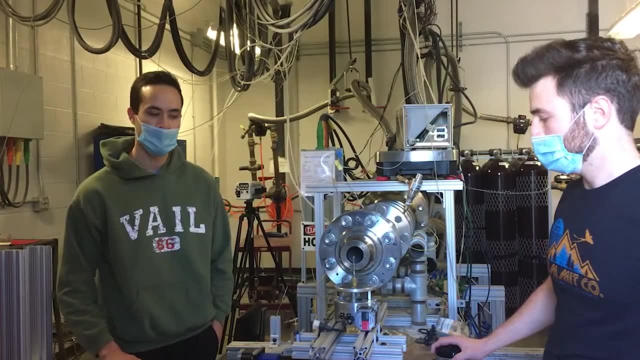 We're going to be filming everything so that we can see how our probe holds up And also see. we're going to be using a flow meter to measure the volumetric flow rate that's being captured by the probe And we're basically going to be using the camera to make sure that that flow meter works correctly. 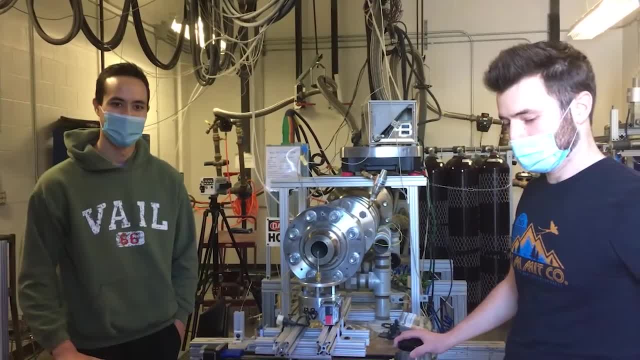 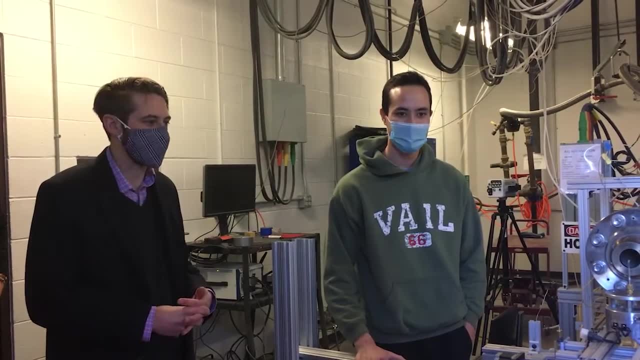 And so, overall, we just want to make sure that we know what we're doing. Yeah, I just want to add that this project is really important for some work that we're doing for the Navy, for the Office of Naval Research, where we want to understand the impacts that particles have on. 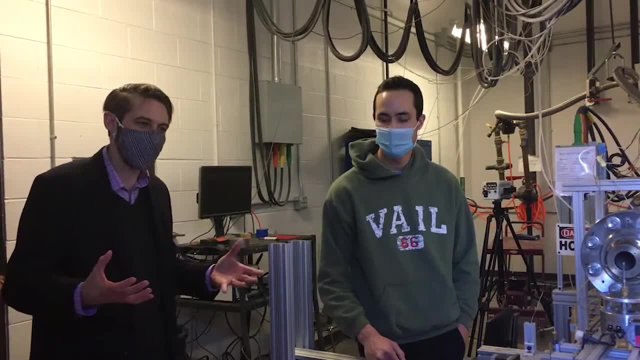 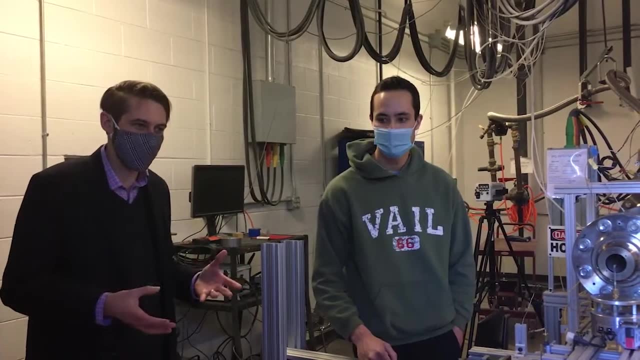 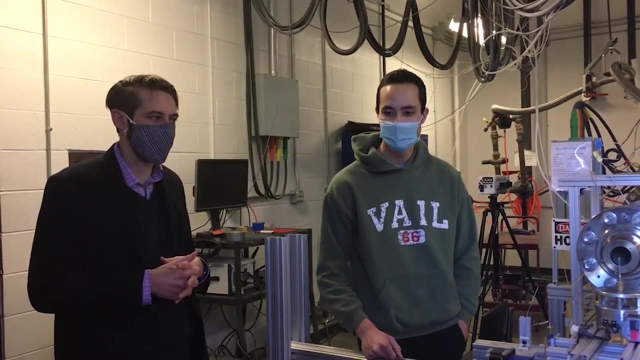 the performance and the reliability of jet engines. So there's turbo shafts and turbofan engines- And to help these engines to have longer lives and have less cost to the Navy And then, most of all, to avoid catastrophic failures of engines in the field, 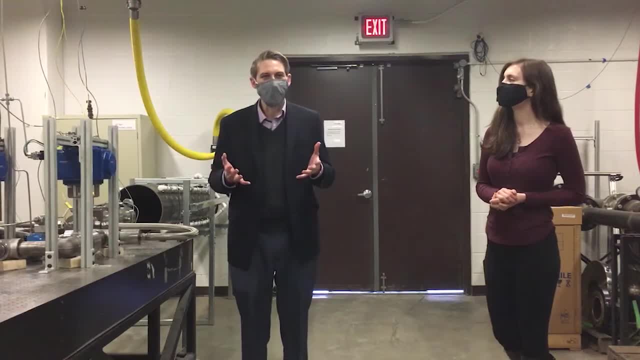 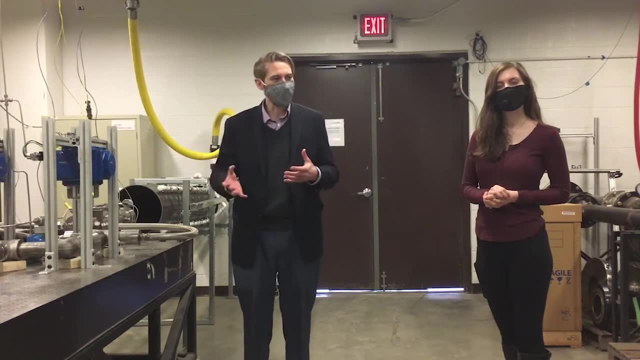 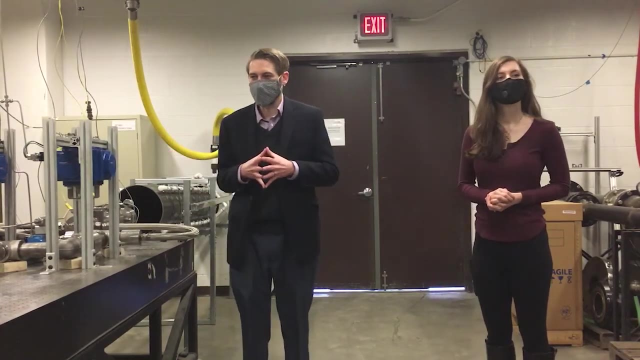 We're now in a combustion cell, And so this is where work that goes on. I know we're doing hydrogen, or usually hydrocarbon combustion. There are two major rigs here. The one that you can see now that I'm standing beside of is a really 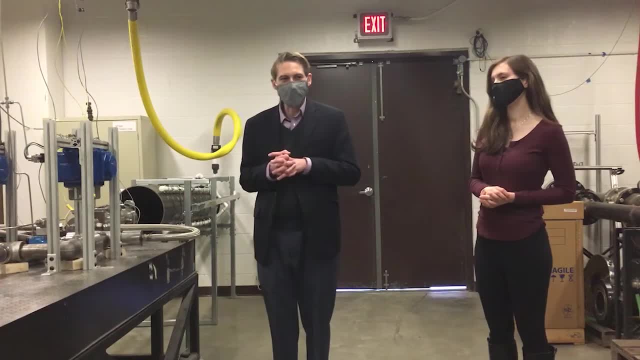 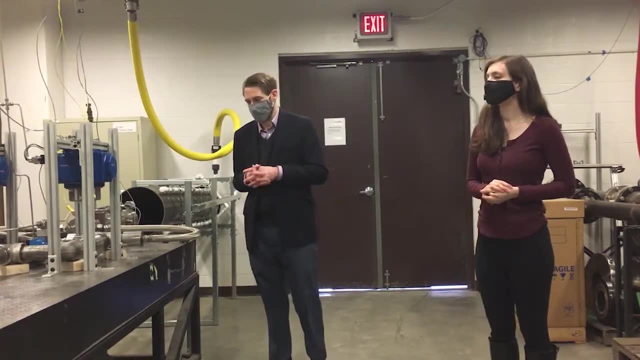 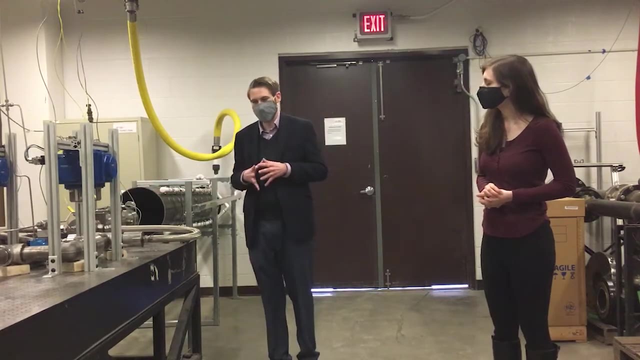 interesting and very new rig. It's a solid fuel ramjet simulator, So a ramjet engine simulator that has been designed by Dr Young's group and built and now is being commissioned. So the actual business part of this is happening right down in this tube And this is work. 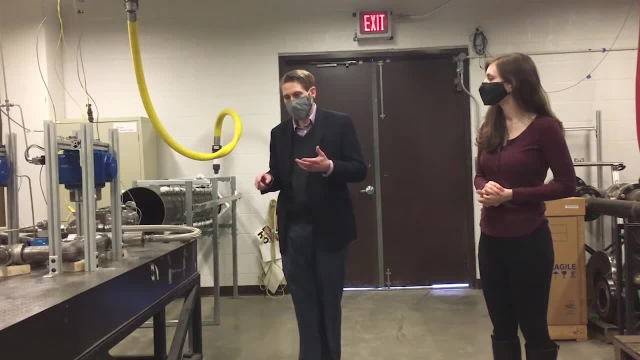 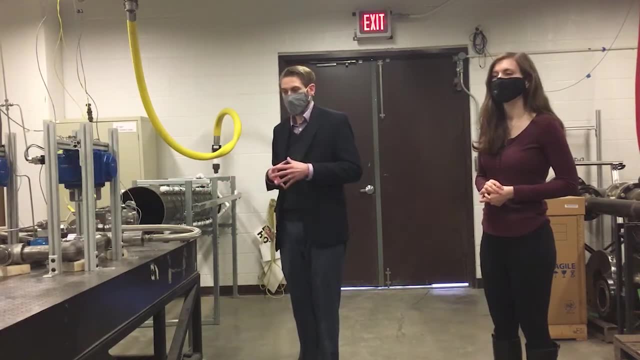 that they're trying to understand some of the fuel properties and combustion properties of solid fuel and link that to the performance, stability, reliability of ramjet engines, And so it's really pushing the state of the art for what we understand for these sorts of. 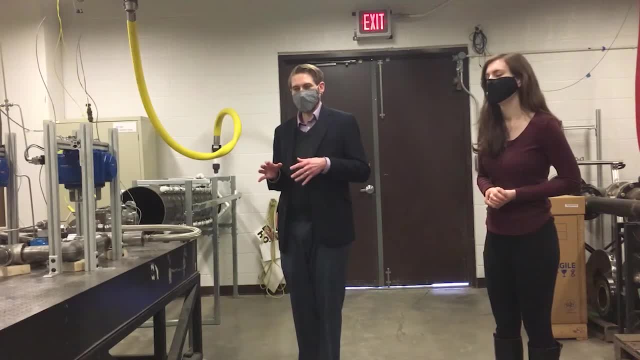 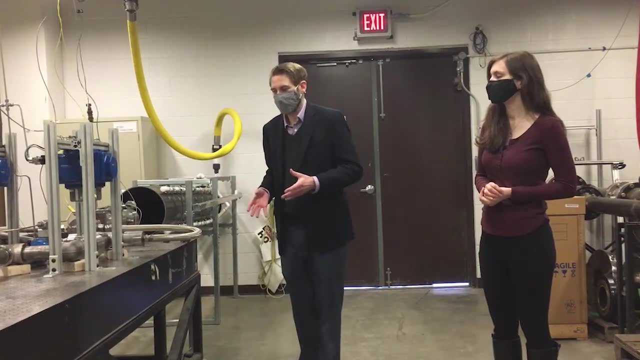 systems. One thing I did want to point out with this rig. I think it again highlights their philosophy in this laboratory, which is to have modular experiments. If you were here two months ago, you wouldn't have seen anything beyond about this. the 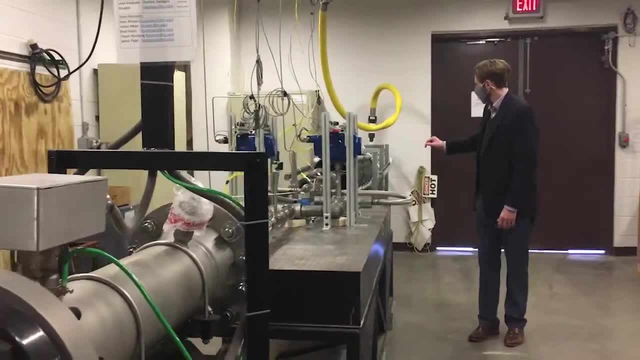 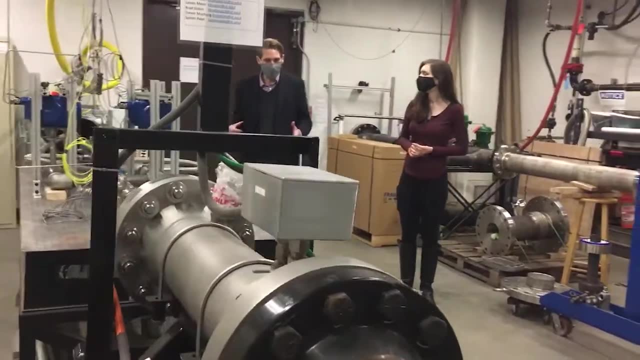 coupler. that's kind of right there, And so all of this has been built. We actually modified the way that the rig exhausts outside, And all of this is now ready to be up and going. If you were here six months ago, there was an